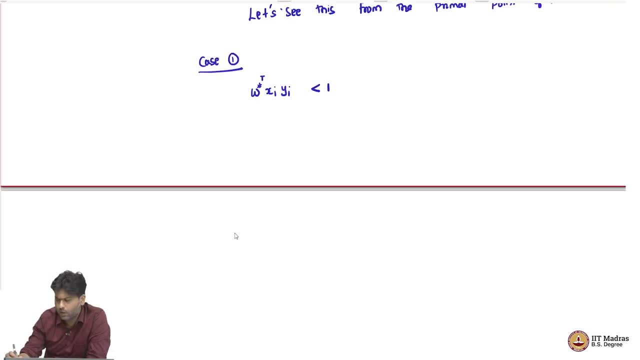 be a point which is misclassified. Now, what can we say about this, right? So the moment I observe that this happens, what can I say? Well, I know that, from my feasibility, W star transpose xi plus psi, i star is greater than or equal to 1.. Now, this means that W star 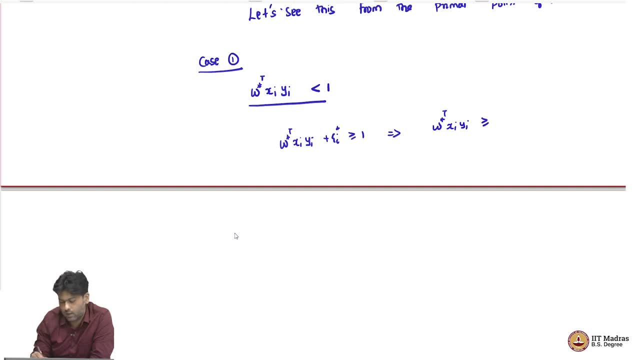 transpose xi yi is, or rather, let me put it the other way- psi i star is greater than or equal to 1 minus W star transpose xi yi. Now this implies that we are assuming that the point satisfies: W star transpose xi yi is strictly less than 1, that is the case. 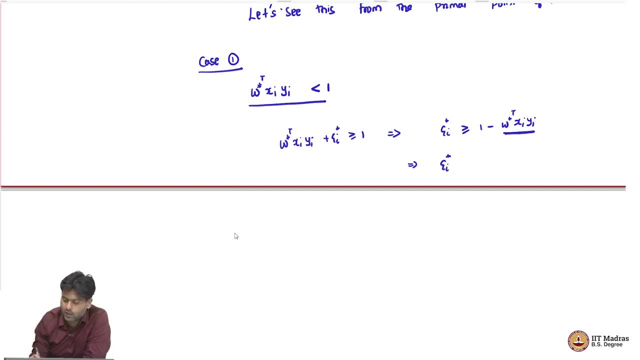 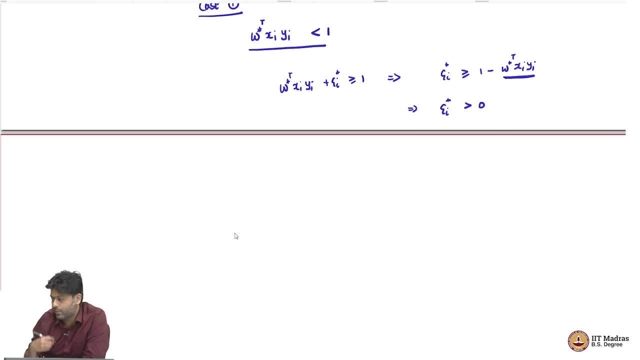 we are in Now. this means that epsilon i star is strictly greater than 0, because this guy is strictly less than 1, the whole thing has to be strictly greater than 0.. Well, if epsilon i star is strictly greater than 0, now by complementary. 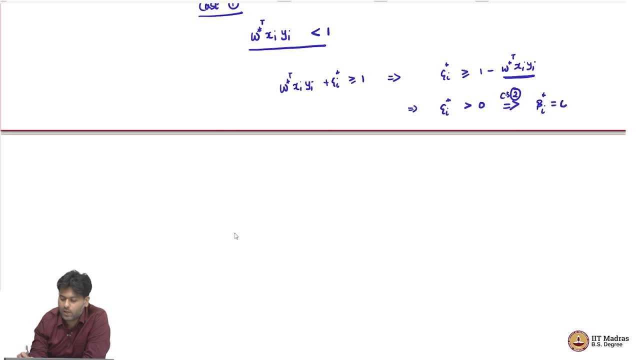 slackness 2, we know that beta star i will be equal to 0, because the product has to be, the product has to be equal to 0.. Now, beta i star equal to 0 implies alpha star i equals C, right, So now what is this saying? This is saying: 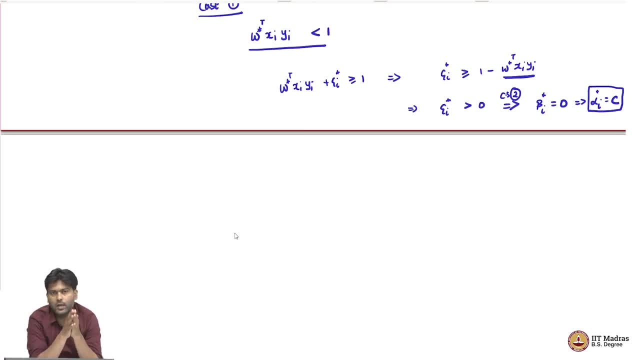 that if I solve the primal and I find that a point has strictly less than one margin, then it means that that point necessarily has alpha star. i equals c, right? So I am not saying the point is lying on the hyperplane, the point is strictly away from the hyperplane. 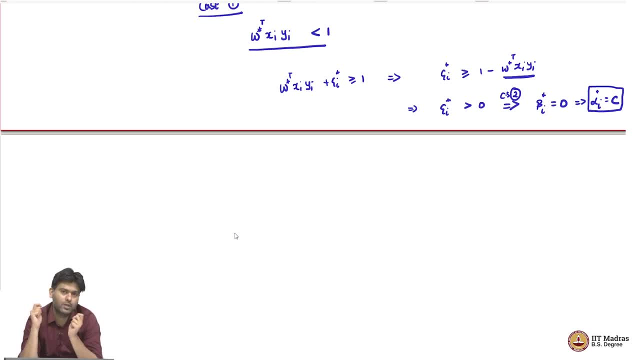 but on the wrong side. then that point is very, very important because alpha star i equals c. for that point, that is the implication that we, that we derive here The other cases. case 2 is when w star transpose x, i, y, i equals 0.. Now, if I solve, sorry, equals. 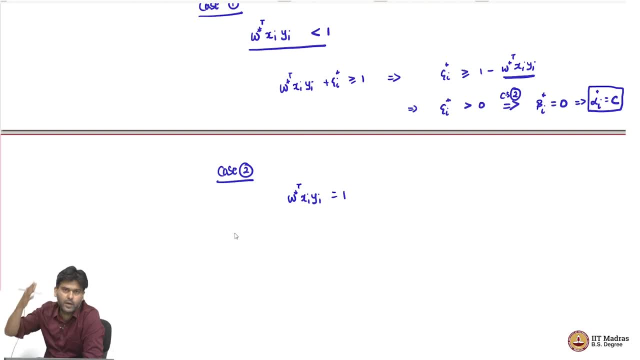 1,. now if I solve the primal problem and I observe that a point actually lies on the supporting hyperplane, can I say anything? Well, I know that epsilon star i is greater than or equal to 1 minus w star i. transpose x i, y, i by feasibility, then I can say that: 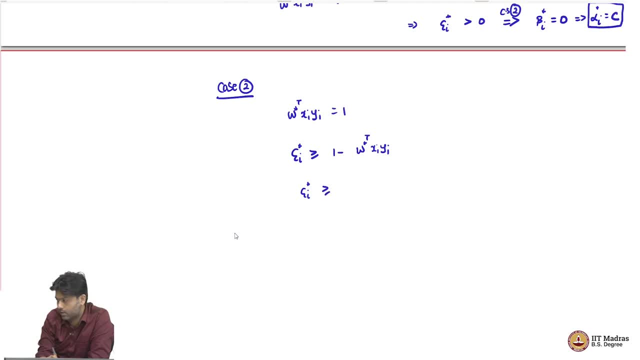 but now this guy is 1, which means that epsilon star i is greater than or equal to 0,. I cannot really say anything more from this argument. Well, this just implies that alpha star i belongs to. well, I cannot say anything about beta. 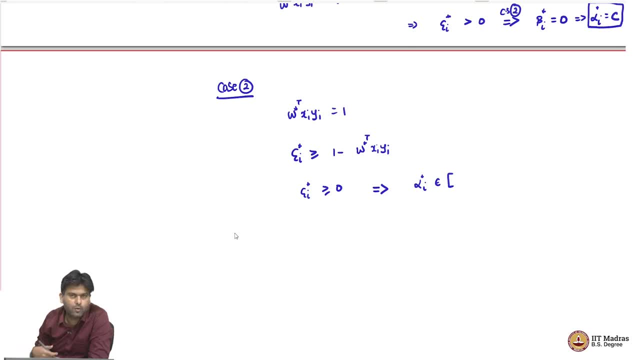 If epsilon star i is greater than or equal to 0, beta can be greater than or equal to 0,. if beta is greater than or equal to 0,, then alpha has to be between 0 and c, right, So I cannot really take away any specific values for this alpha, which means that if 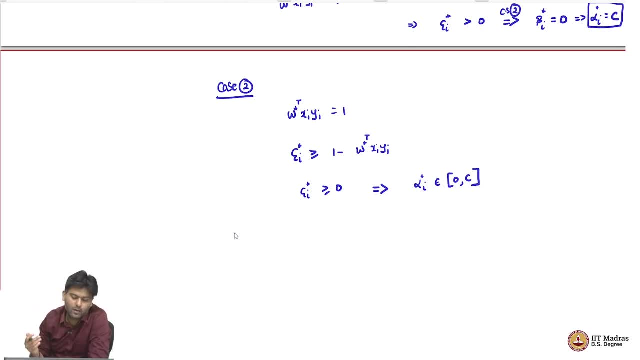 the point is on the supporting hyperplane right. so then alpha star could be anywhere between 0 and c. It could be 0, it could be c. it could be anywhere between 0 and c. From the previous argument we said that if it is between 0 and c, if alpha star i is. 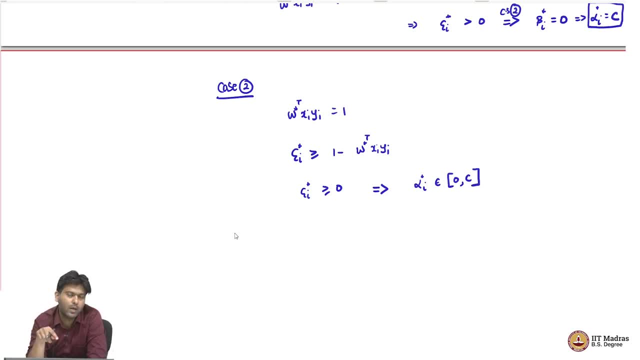 between 0 and c, then I know that it has to be on the supporting hyperplane. But then if I find a point on the supporting hyperplane, well it does not imply that alpha star i is between 0 and c. that is not an if and only if. that is what I am trying to say. If you, 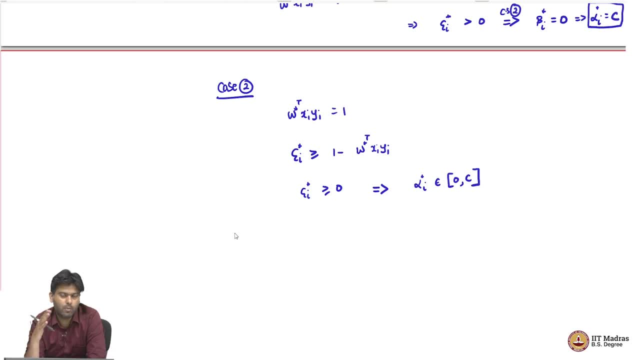 if you solve the primal problem, then you will have ejercised the probability Whiskey's and you observe that a point is on the supporting hyperplane, then it you can only conclude that alpha star i can be between 0 and c. that is the second case. 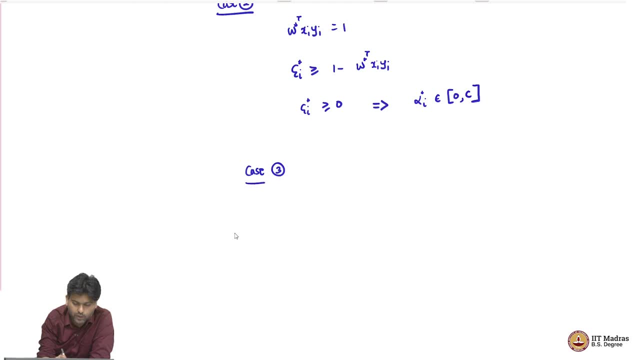 The third case is the good points, where w star transpose x, i, y, i is greater than 1, which means the points for which you know you are classifying this with margin greater than 1, which are like well away from your supporting hyperplane. Now, this implies what? 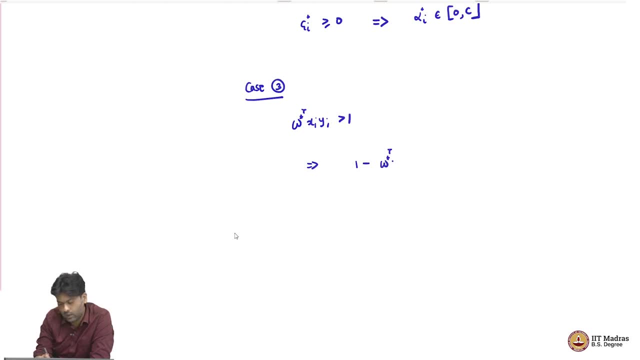 Well, this implies 1 minus, you know, w star. transpose x, i, y, i minus epsilon star i. what can we say about this? Well, if this is greater than 0, well we can conclude that, well, this guy is less than 0,. but because epsilon star i is greater than or equal to 0,, well we can. 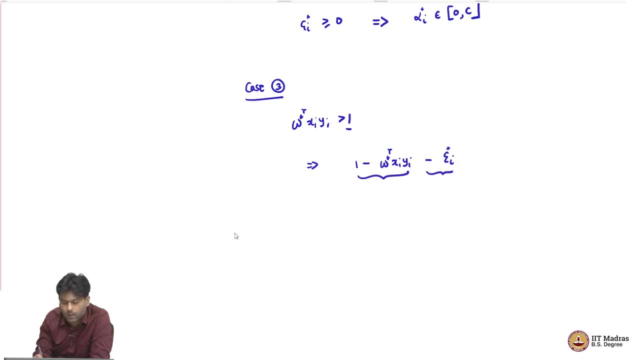 say that this is a negative quantity. Now, this can be 0 or negative, and so this whole thing is strictly less than 0.. Well, whole thing is strictly less than 0, now, by complementary slackness 1, we can conclude. 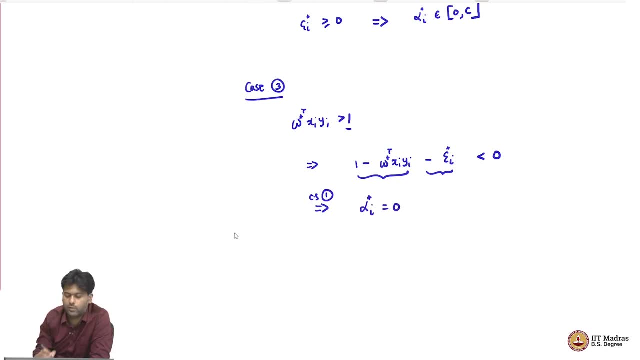 that alpha star i has to be 0. Well, what does this tell us? This tells us that those points which are classified with margin strictly greater than 1 do not matter. they do not really, you know, are part of this support or part of this W star. they do not contribute. 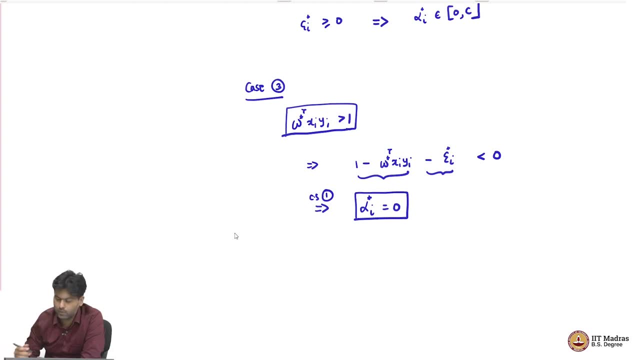 to W star. So that is the conclusion that we are able to derive. right? So this is from the primal point of view. Now let us just summarize all of this to see everything together so that it becomes much clearer. The summary is the following: right? So if I start looking, 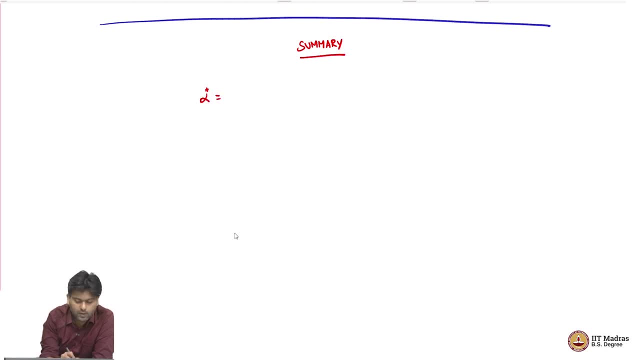 at it from the dual point of view, there are three cases: alpha star equals 0, 0 and alpha star is between 0 and c and alpha star equals 0. So if I look at it from the dual point of view, I have W star transpose. sorry, primal. 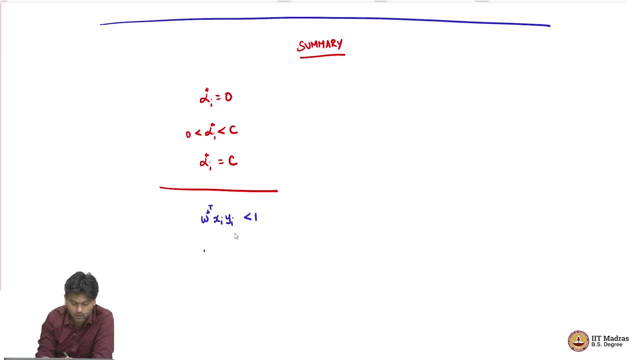 point of view I have: W star transpose x i, y, i is less than 1, W star transpose x i, y, i equals 1 and W star transpose x i, y, i is greater than 1.. Now, this is what we saw is. 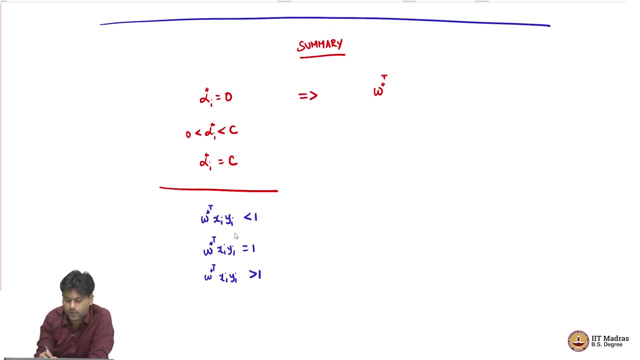 that if alpha star i is equal to 0, this implies W star transpose x, i, y, i is greater than or equal to 1. So it is classified with margin at least 1.. If you find alpha star i is between 0 and. 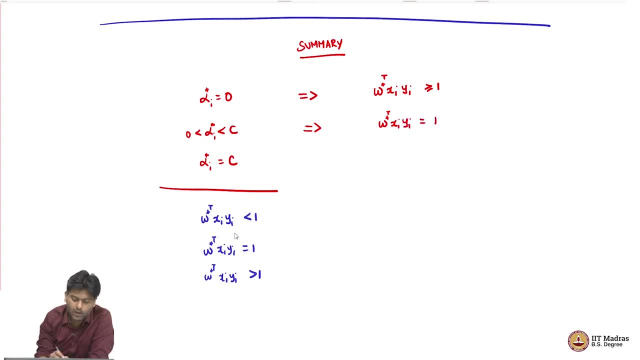 c, then it is exactly on the hyper plane, and if you find alpha star i equals c, then it is classified with margin less than or equal to 1.. On the other hand, if you find a point which is which has strictly less than 1 margin, then that implies alpha star i equals c. If 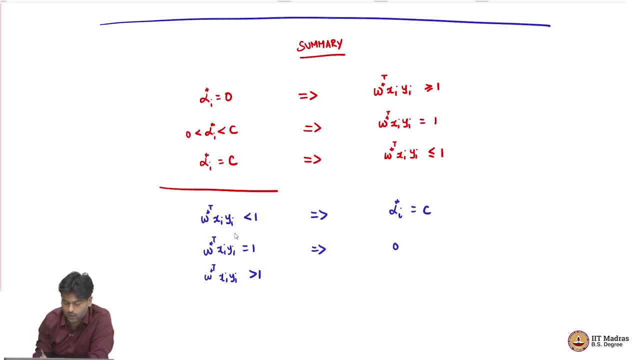 a point is on the hyper plane, then you cannot really conclude anything about alpha star i. and if the point is away from the hyperplane in the right way, then alpha star i does not contribute anything right. So the does not contribute anything to our, to our final data. final conclusion: W star. So this is the summary. 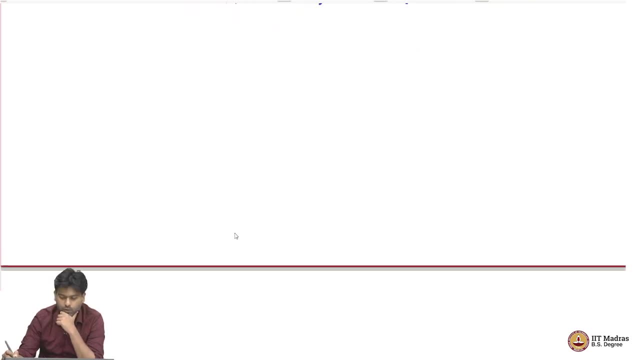 So, so, just to give a feel for in pictures, right? So let us say we have a data set like this. yeah So, let us, let us say: this was our W star. now, if I told you that this is my W star, well, this is, these are the supporting hyperplanes. let us say: this was my data set. 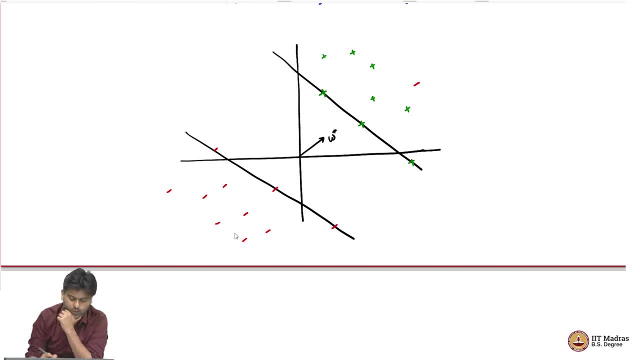 bunch of points this side, bunch of points on the line. maybe that is a point here. let us say: this was our, this was my data set. Now, if, if you are asked the question, if this is the scenario, and let us say, I solve the problem and I observed the W star is like this. now, if I ask the 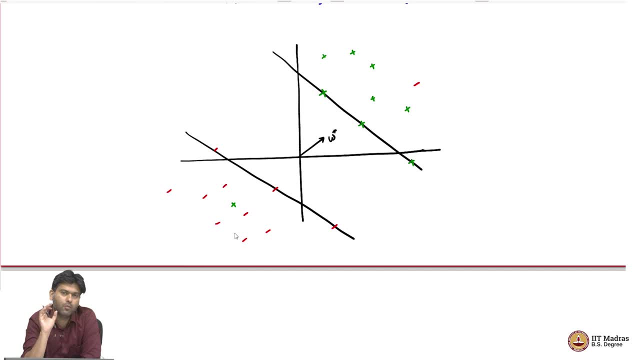 question. well, what can I comment about the which are the important points, which are the support vectors? well, what can I say? right, So I can go over each of the points and see you know what equation does it satisfy with respect to W star? Now, this is W star transpose. 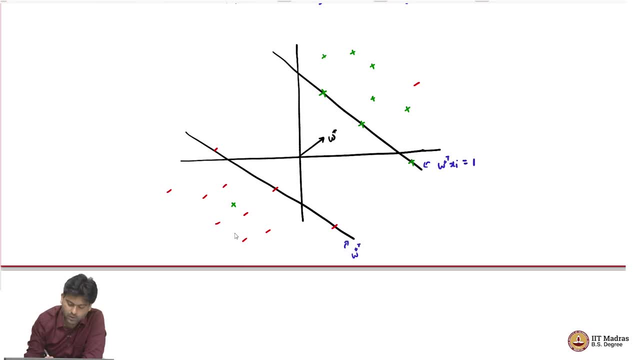 x i, y, x i equals 1,. this is W star transpose. x i equals minus 1.. Now, if you look at this, these points, right so, which are labeled with margin greater than 1, or these points which are also labeled with margin greater than 1, right So these are on. I mean, these are not on the 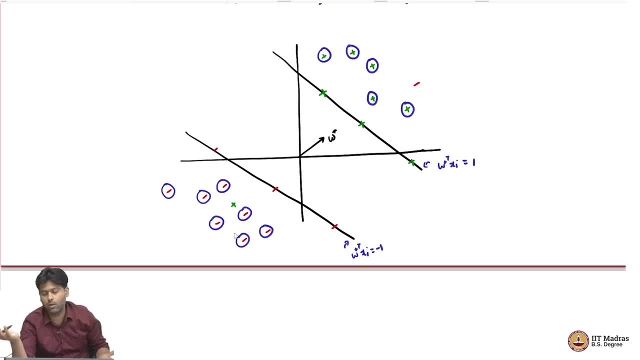 supporting hyperplane away from the supporting hyperplane and is classified correctly. also, these points right? So any point like this does not contribute to my W star at all, right, So alpha star is 0.. Now, if I look at these points right, so this, this plus and this minus. 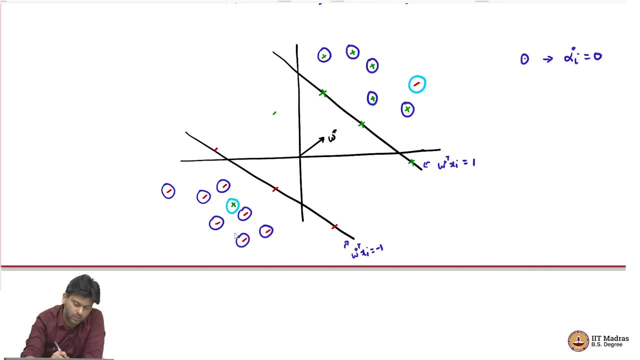 right Now. maybe I should add a point here as well. maybe I will add a point here and as a plus point. Now let us look at these. these three points maybe right, So I can include this point as well in the discussion. or maybe there can be a minus here also, right? So these four. 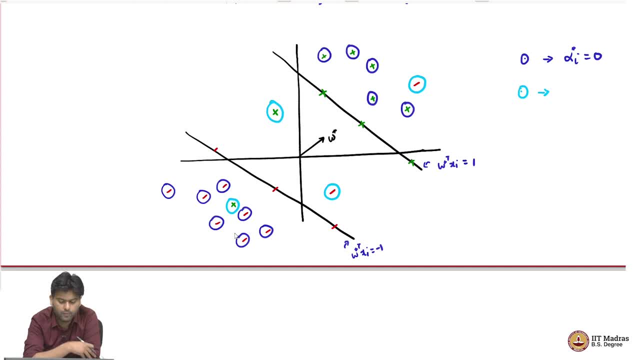 points. now, what can I say about these four points? Well, for these four points, W, star transpose x, i, y, i, which are as these 4 points. we are adding points here like w into x, i, r into x, i, minus and minus here, my phi right, So rho of y to that, So rho of y to that. 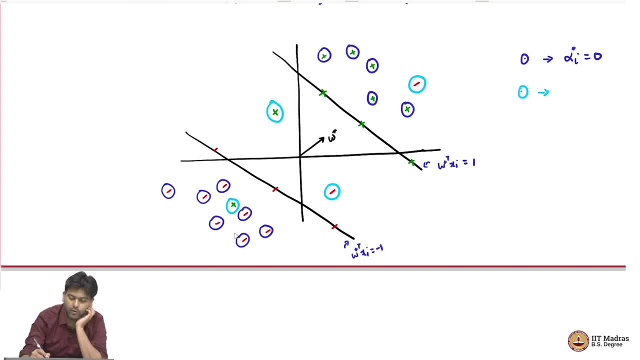 y to y minus, So rho of y to that means phi over y and the extra, the touched points above right yi is strictly less than 1 right. So in fact, for the points where I am pointing with the arrow w star, transpose xi yi is actually less than 0, because they are incorrectly classified. 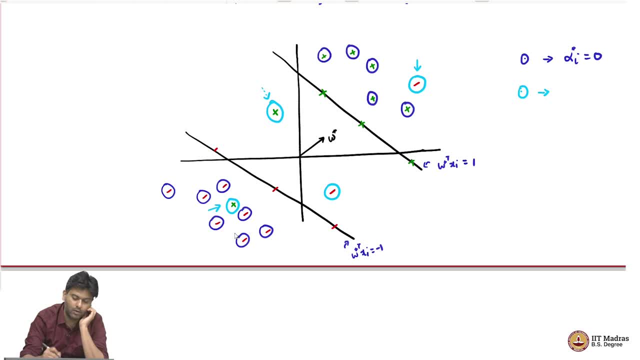 by w star, whereas the points which are where I am pointing with dotted arrows, these are correctly classified by my w star, because w star is eventually going to classify using this line, right? So the dotted light blue arrow points are correctly classified by w star, but then they are not classified with enough margin. So 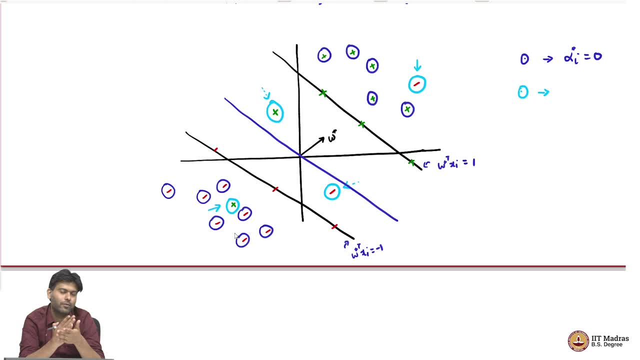 it does not matter if it is correctly classified or not, as long as it is not classified correctly, classified with enough margin. all these points are contribute. you know similarly and then, in fact, they are the most important points. for these points, alpha star equals c. Now, 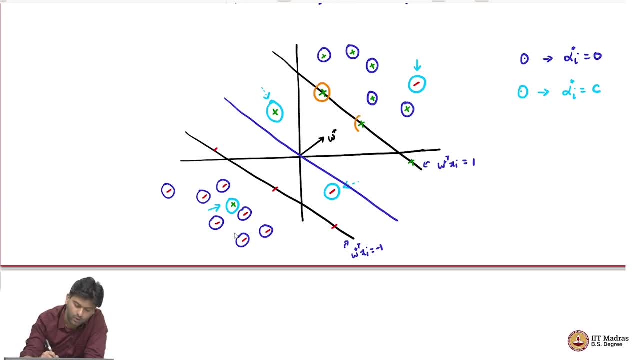 there are some more points which I am going to you know, highlight using orange circles. So, these points, What can I say about these points? Well, they are on the supporting hyper plane, right? So if they are on the supporting hyper plane, I cannot really conclude what is their alpha. 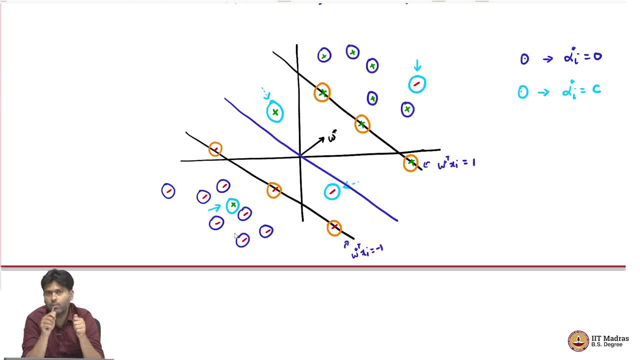 star going to be right. So their alpha star can be anywhere between 0 and c. what I can conclude is that if I know that for a point alpha star is between 0 and c, then I know that it has to be on the hyper plane. 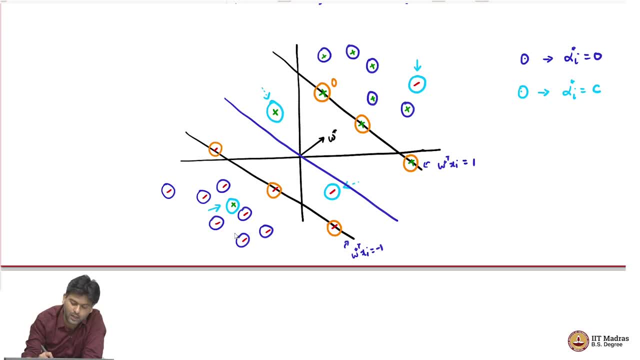 But it should. it could so happen that this guy has alpha 0, this guy has maybe 1, this guy has c. let us say, c is greater than 1, this guy has 0, this guy has 1, this guy has c. 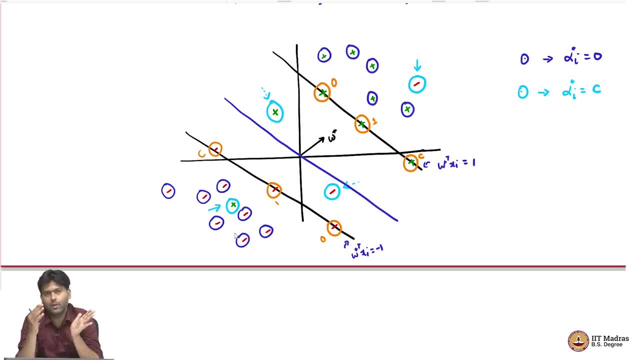 all sorts of things are possible here. So on the line, it could be either 0,, it could be c, it could be 1.. So, but the moment I say that for this point, so 1, the value is 1, which is. 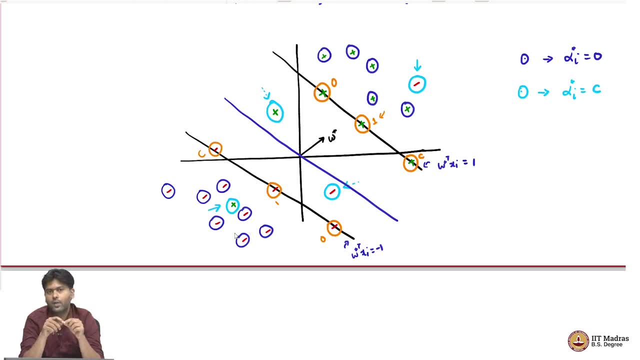 between 0 and c, Then I know for sure that this point is on this line. So these two points are on this line. but if I just say that the point has value 0 or c, then I cannot really conclude it is. 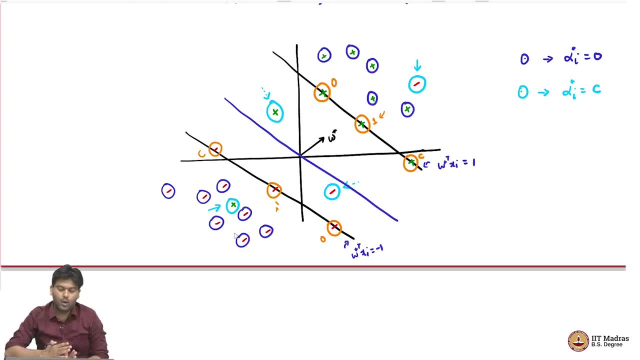 exactly on the line. So on the line can take any value. on one side of the line, you get exactly 0 values. on the other side of the line, you get exactly c values on the line. it can be anywhere between 0 and c. That is the conclusion that we draw here. Now the final point that I 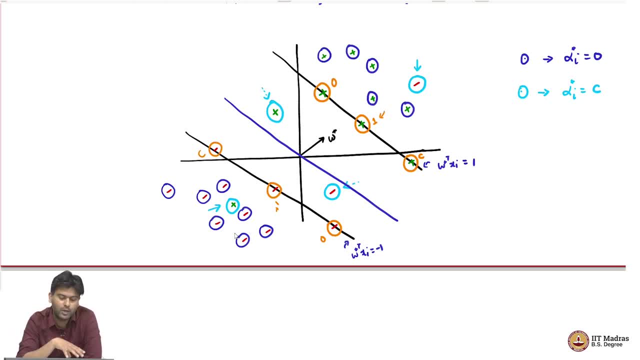 want to draw here. so I am going to draw the solution that I am going to draw here. so I have written here in the first two sections and then I am going to draw the solution Now. the final point want to make about this is that, still, if you look at this, picture everybody. So let me 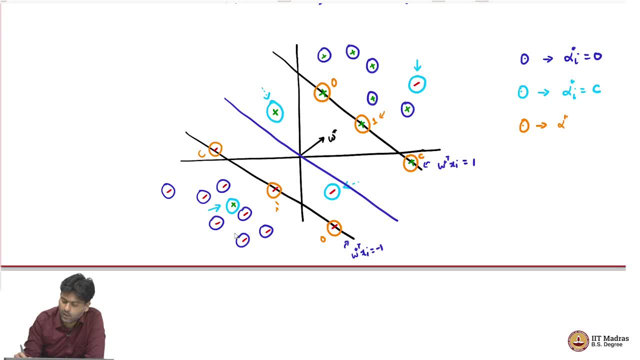 let me point this right. So this, this points: can alpha star, i can belong to 0 and c, I do not know right. So it can be anywhere. So the final point that I want to say is that, still, if you look at the number of points which are actually going to contribute to, 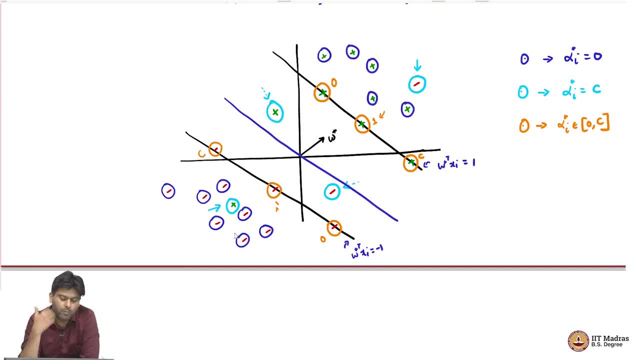 my w star they are. they are going to be only a handful because all the points with blue circles, dark blue circles, I have kind of. I know for sure that they are. their alpha star is 0. So they do not contribute to my w star, The only ones that contribute to my 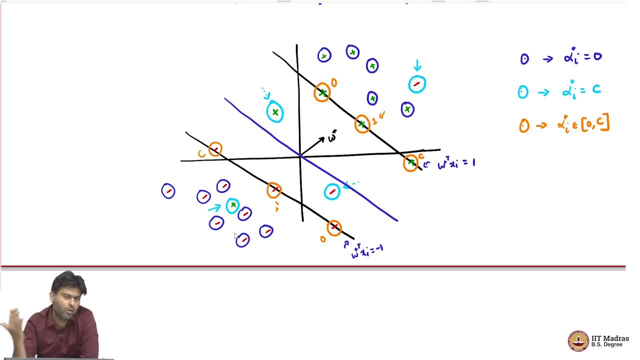 w star are either on the hyper plane supporting hyper plane or on the wrong side of the supporting hyper plane. This, the hope, is that this set of points is still going to be a small set as compared to the billions of data points that we might have right. 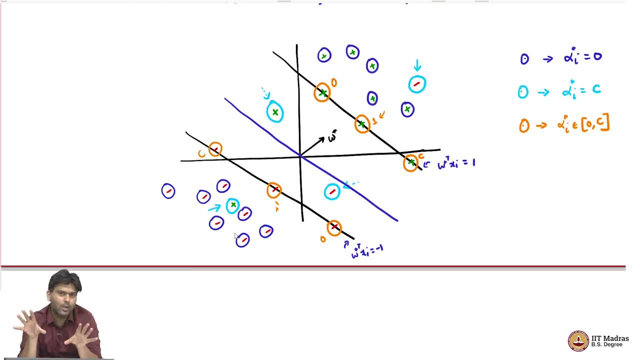 So, because if your data set is indeed linearly separable, with some outliers with respect to you know, Whatever kernel that you are using, then it is, you are still going to get a good w star where you the points which are not, which are either on the supporting hyper plane or 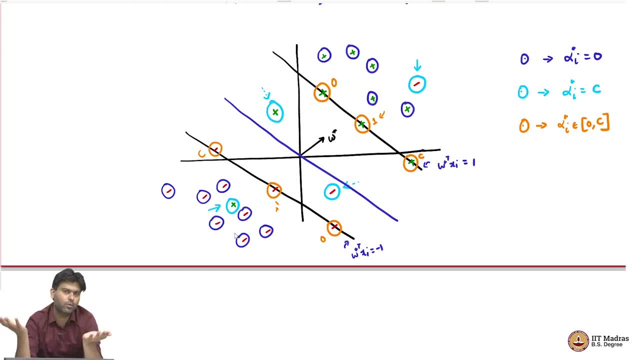 on the wrong side of it are going to be much smaller in number compared to the total number of data points. So you still are going to get a sparse solution, which means that the conclusion is that, even with respect to sparsity, the soft margin support vector machine does. 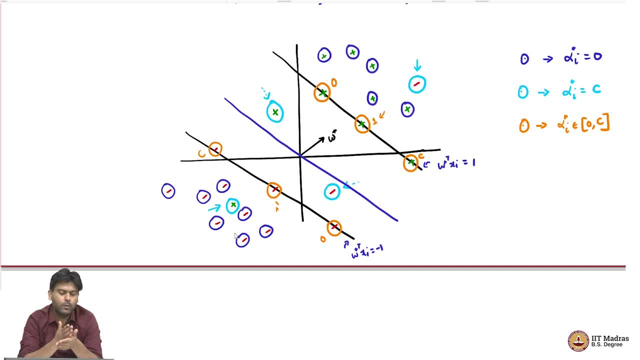 not lose out anything. that is the final conclusion that I want to draw. So to summarize our discussion About soft margin support vector machine, by looking at the dual, we are saying that it can be kernelized, point number 1.. The constraints for alphas are very simple. these are box constraints. 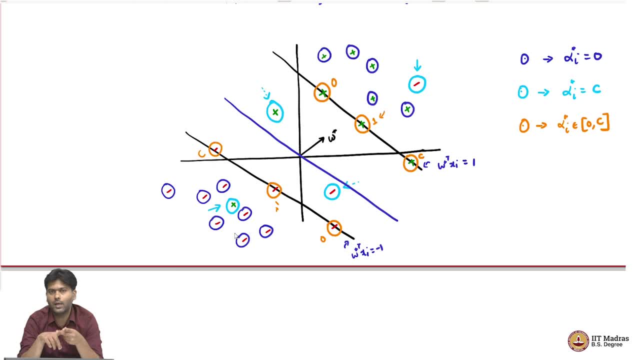 between 0 and c, which are easy to handle, even if you are doing like a projected gradient descent kind of algorithm. And the final point is that you know the solution is still going to be sparse. that is the number of points for which alpha star i is not. is is going. 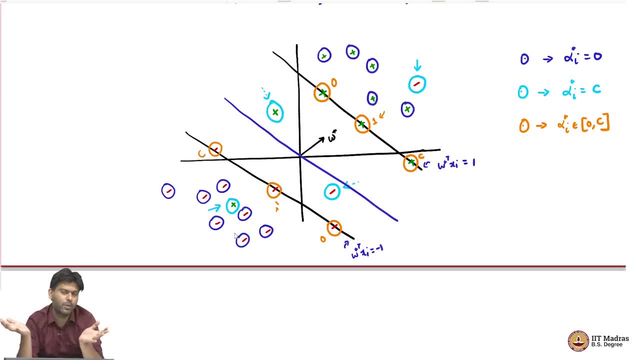 to be non zero is still going to be a handful of points when compared to the total number of points that you have. So all these make the soft margin support vector machine as super powerful, elegant formulation and and that is why you know it is. it is not. 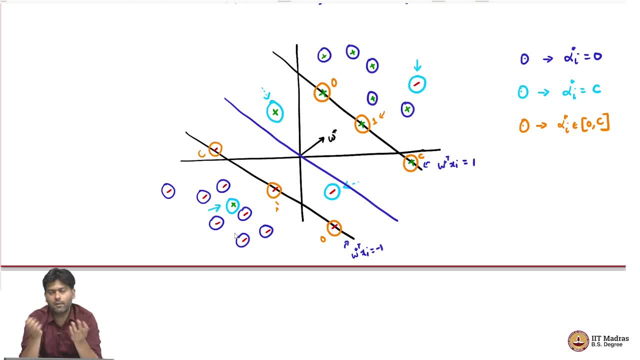 just the theoretical elegance. that is why, if you look at several practical applications, this algorithm performs really well in practice. So so, with this, what we have, kind of what we can conclude, is that, you know, what we have seen so far is a very powerful 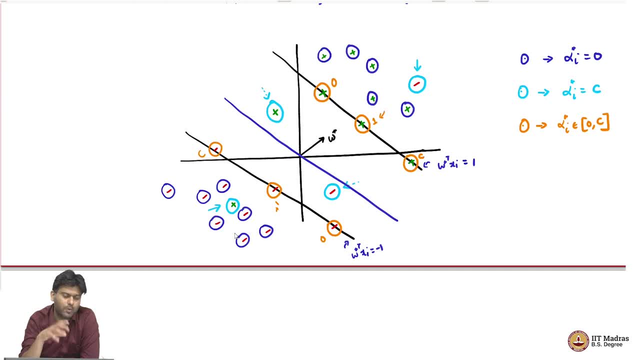 Algorithm in classical machine learning called the support vector machine. we have looked at in quite some detail And- and this has, you know, been successfully applied in several applications, specifically in structured data, that is, data where you have features in a structured format. this algorithm has been, I mean, really found, found to be very useful. 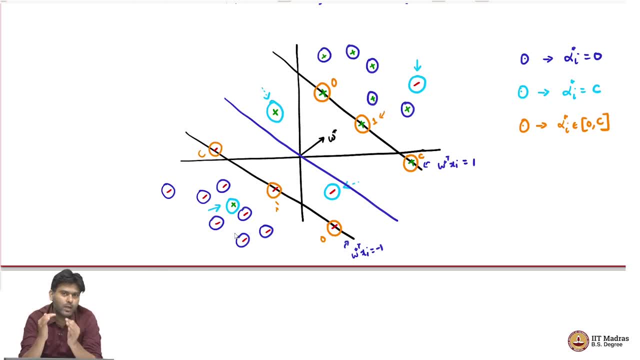 in practice. So the actual implementation of this algorithm. people have worked on a lot of, you know, advanced techniques, optimization techniques to make this implementation really fast. In fact, you can run this algorithm today using the fastest solver which runs in linear time in terms. 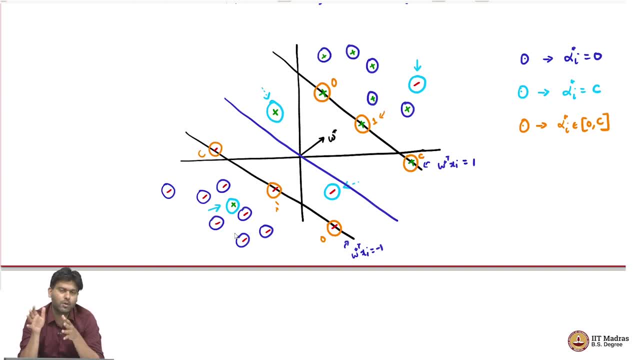 of the parameters of the problem. So, even with respect to the running the algorithm, you know we have very solid optimization techniques which we are not going to look at in this course, but it is good to be aware that you know is because it is a quadratic optimization. 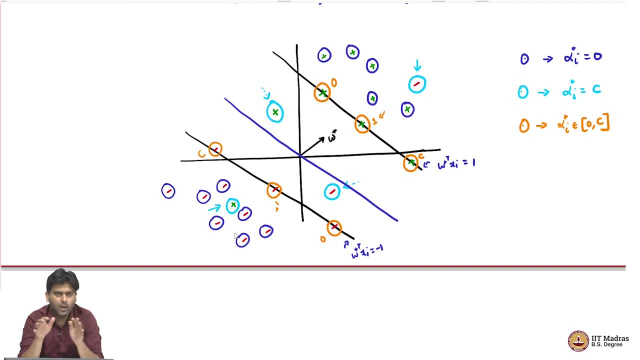 problem, And all of the limits you have to know, is: how much time will it take to solve this problem? it is, it is. it will not take a too much time, typically. So, with all these advantages, we I want to conclude this part of the court by saying: 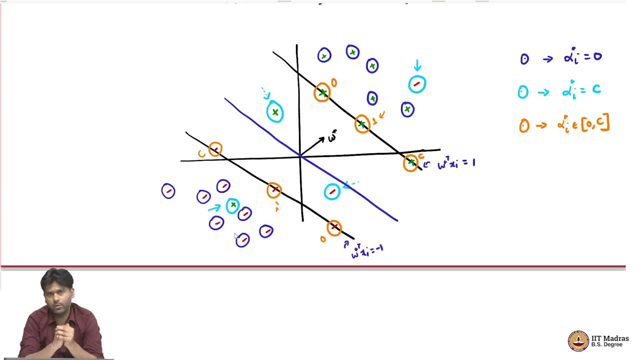 that we we have put down a solid algorithm, which is the soft margin support vector machine algorithm, which can deal with non structural relationships in I mean classification boundaries, decision boundaries, can deal with outliers, it is kernelizable, so it is a very powerful algorithm. So what we are say this, So about a? it only does it. notpie givesきた such an sort.